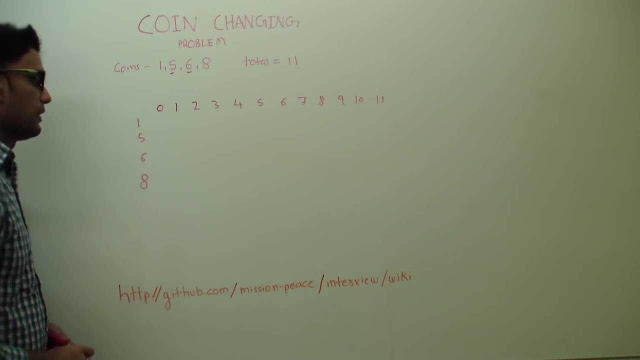 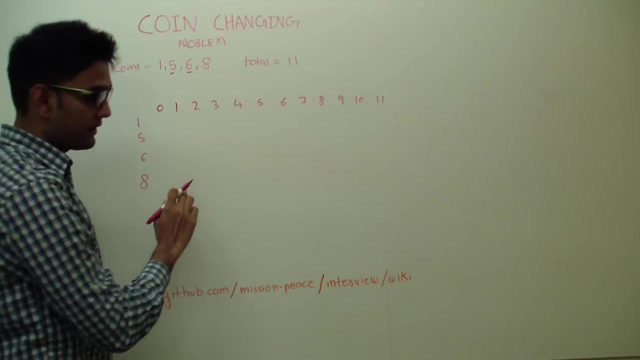 So let's start from 1 and 1.. Okay, Let's ignore everything else. If you have one total and if you have just one coin, how many minimum number of coins would you take to create this 1?? So we know that it's 1.. 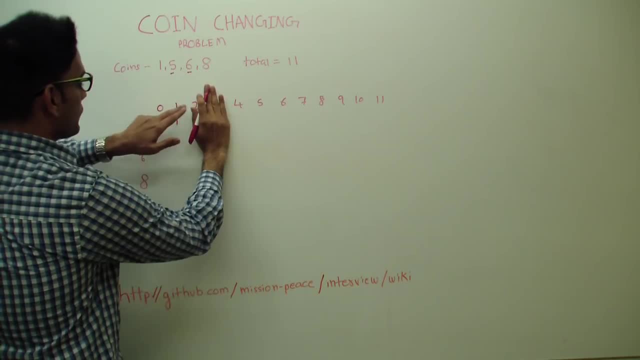 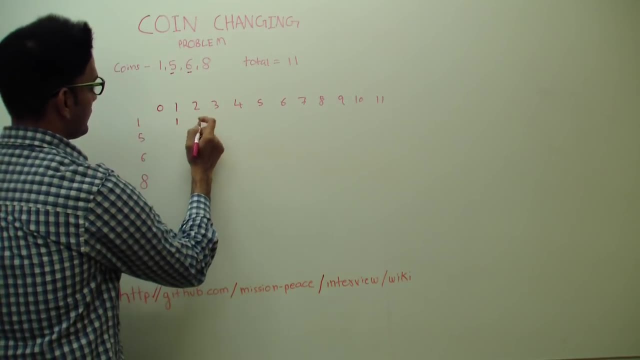 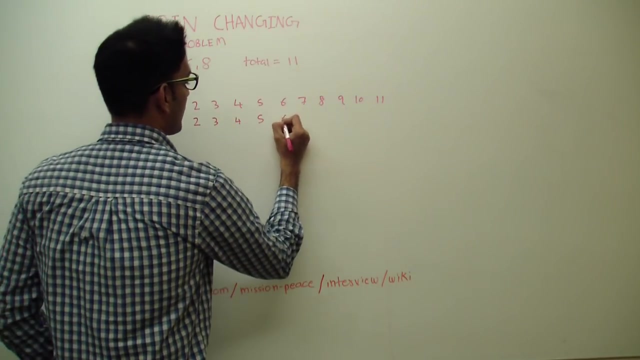 Okay, Let's look at 2.. If you just have two total and if you have just one to work with, how many coins would it take to get 2?? So we'll say 2.. Similarly, we can fill this first row in this manner: 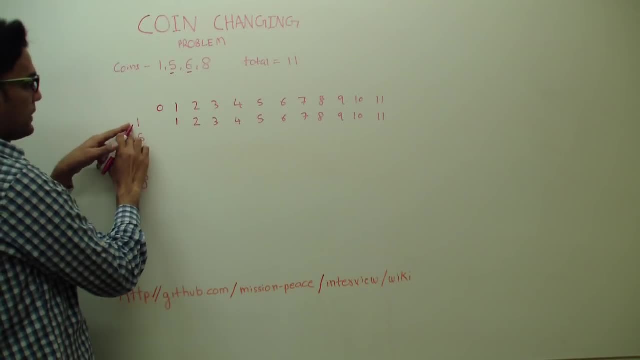 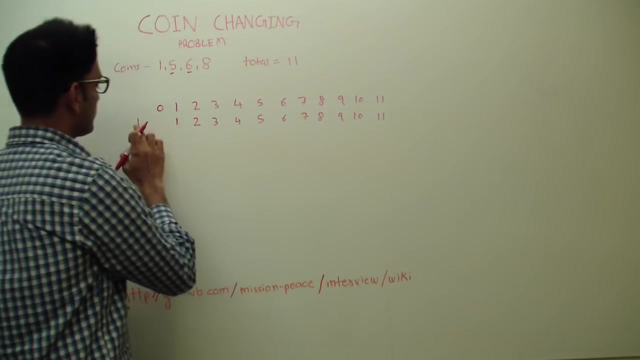 So what it means is if you just had one coin of denomination 1 and if you want to get 11, so we'll need- at least we'll need- exactly 11 coins of 1.. So this is what this first row is presenting. 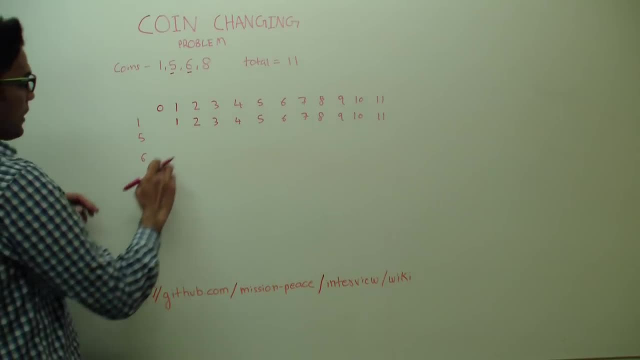 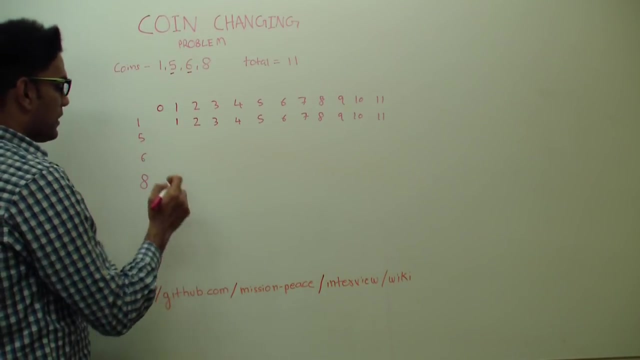 Now let's introduce 5 into the picture. So now we have total of 1. And we have two coins, 1 and 5.. Can we do any better than 1?? I guess not, because 5 is not going to play any role here. 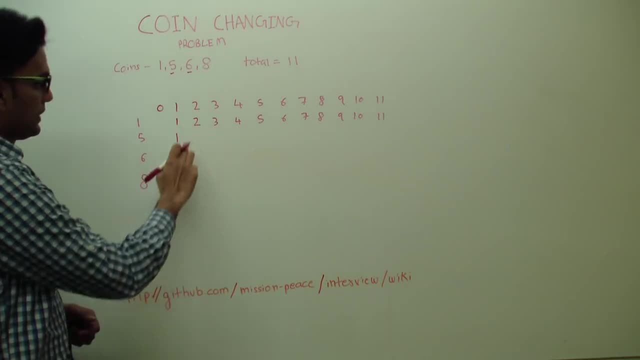 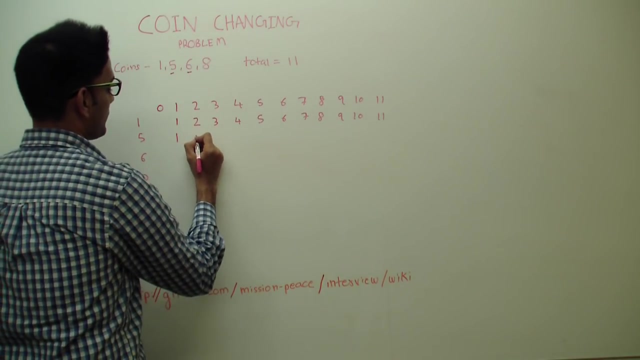 So 1 again. So value is coming from the top. When the total is 2 and we have coins 1 and 5, is 5 going to play any role? No, So value is coming from the top. Similarly, 3 and 4.. 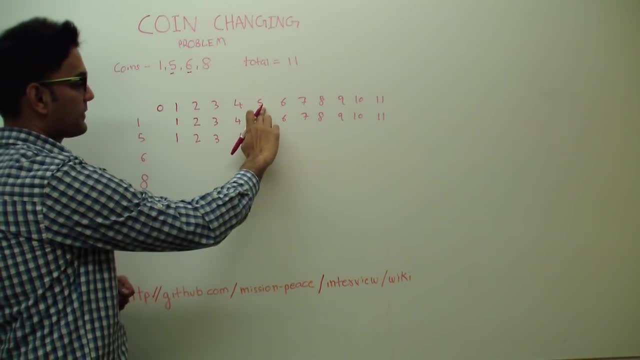 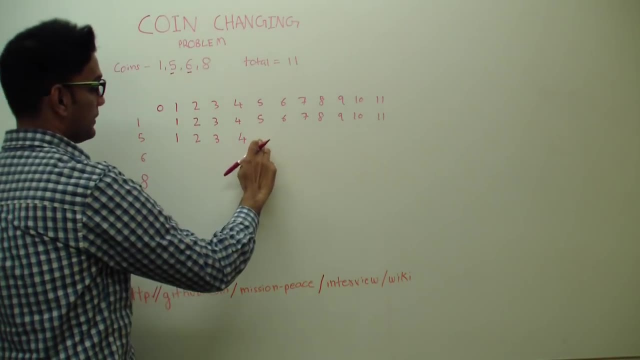 Alright, let's look at 5.. Now, if you want to get 5. And if you have two coins, 1 and 5. What is the minimum number of coins we'll need? We'll not need 5., We'll need 1.. 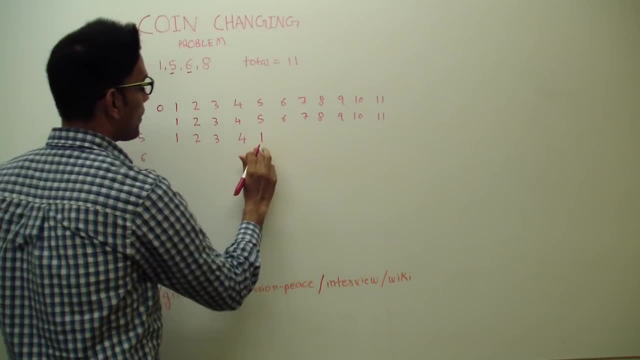 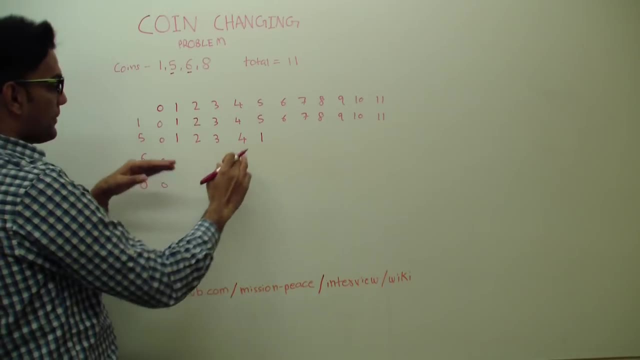 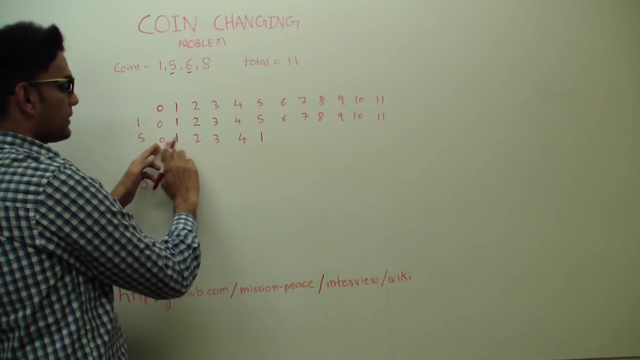 We'll just need one coin of 5.. So how did this 1 come from? This 1 comes from the minimum of the guy in the top, or you go back 5 steps here. So this guy plus 1.. So minimum of 5 or 0 plus 1.. 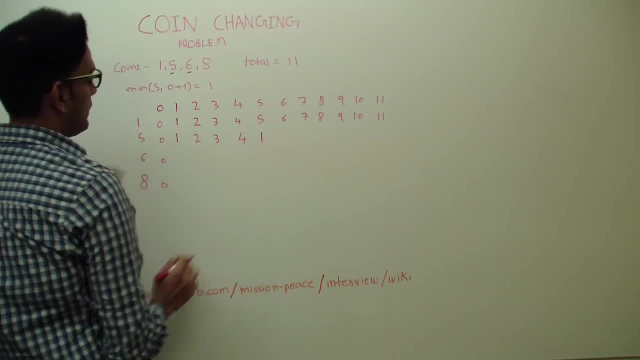 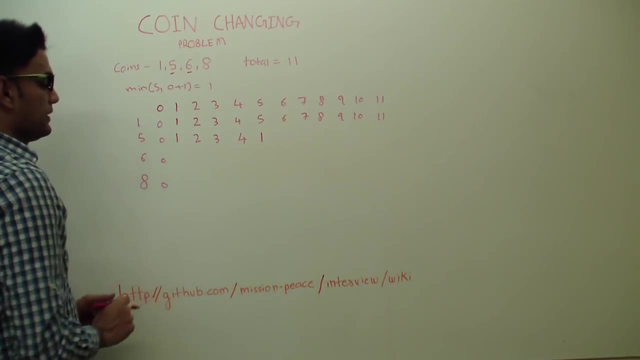 Which is 1.. Alright, let's look at 6.. So if you have to get 6 and you have two coins, 1 and 5, the minimum number of coins you'll need is either 6 or 1 plus 1.. 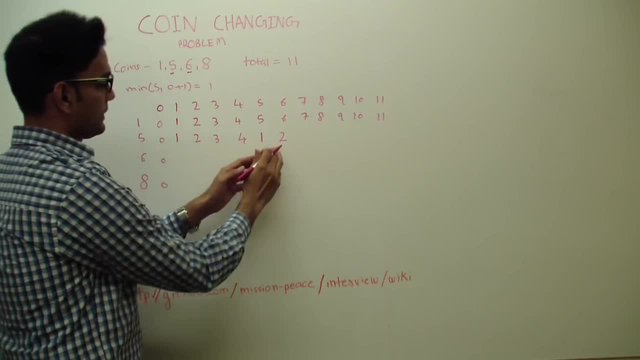 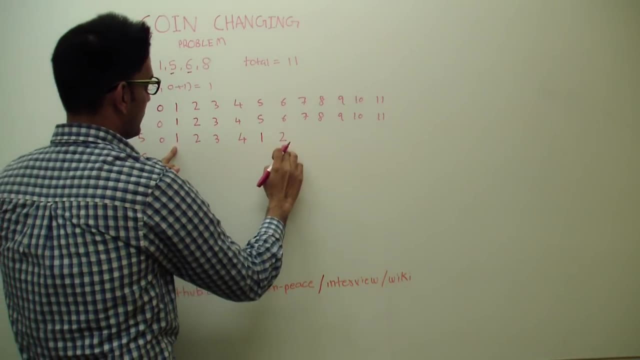 So 2.. So basically, we're going 5 steps back here, So we'll reach at 1.. We add one coin to it, So we reach, So we get 2.. So either 2 or the guy from the top. 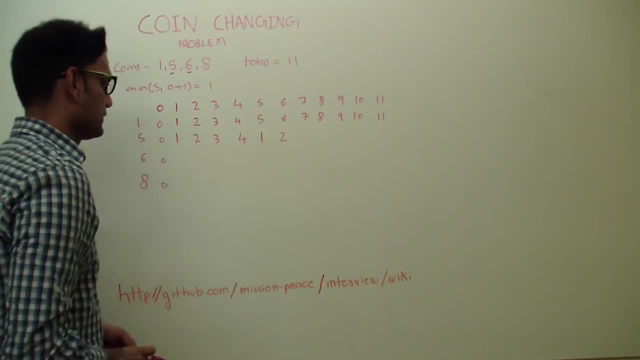 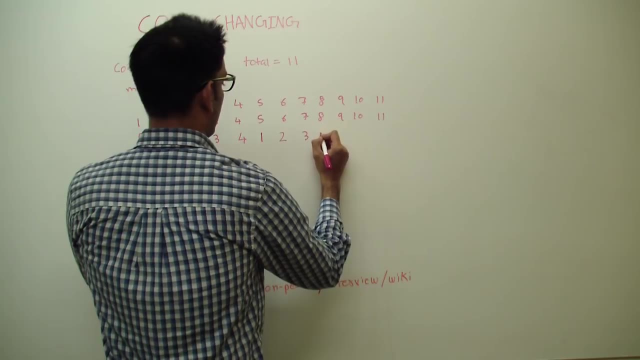 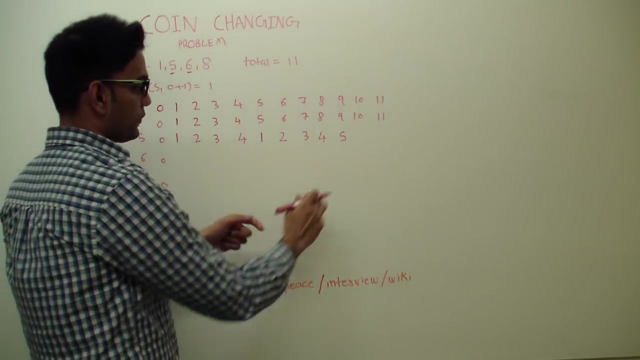 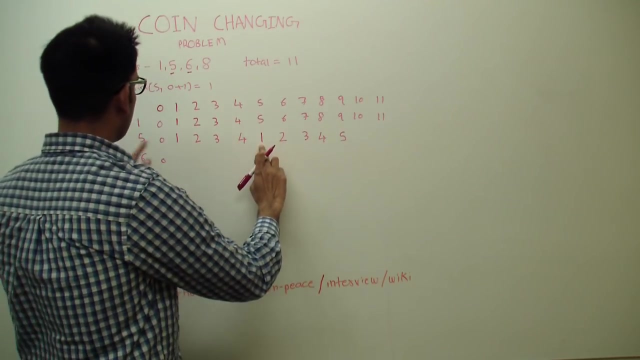 So minimum of the 2, which is 2 in this case, This will be 3., 4., 5. So here, So to get 10, we'll go 5 steps back and we'll be here. So the minimum number of coins will be 1 plus 1.. 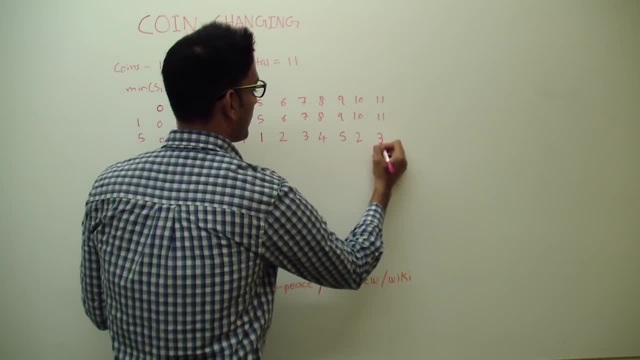 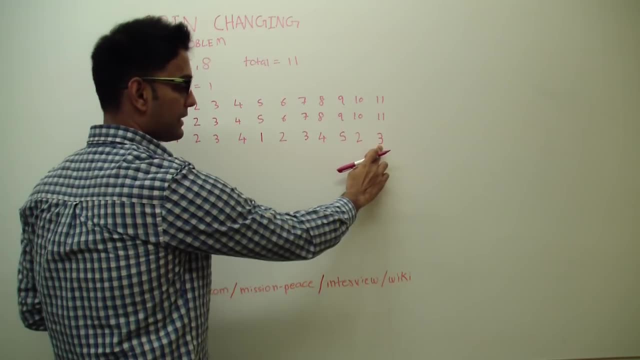 So 2 or 10.. So 2. And this will be 3.. So what it means is, if we have coins 1 and 5 and if we have to get total 11, it'll take us at least 3 coins. 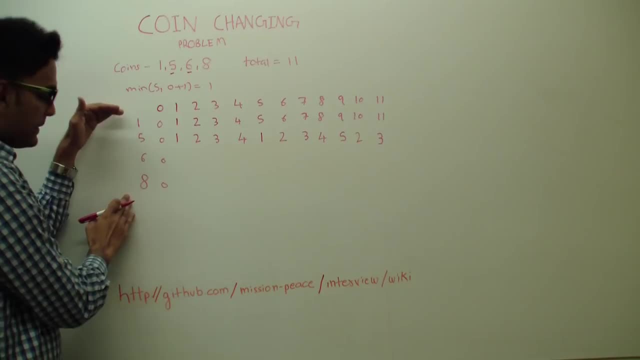 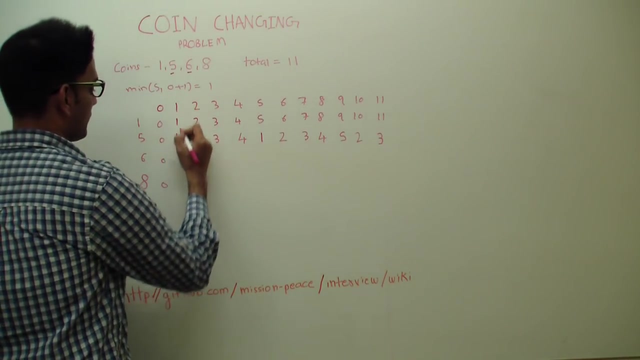 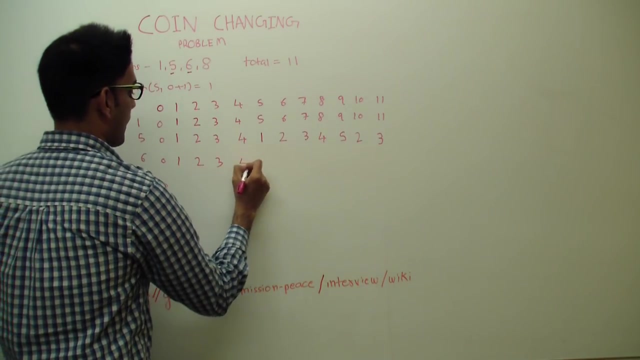 So you see how we are solving the smaller problem. to get the solution for the bigger problem, Let's come to 6.. Alright, So we'll get the values from the top up till 5, because 6 is not going to play any role till 5.. 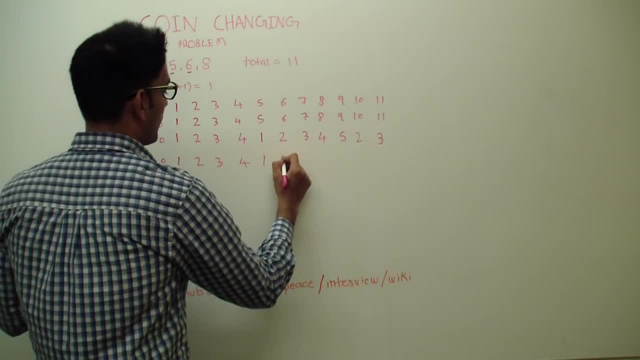 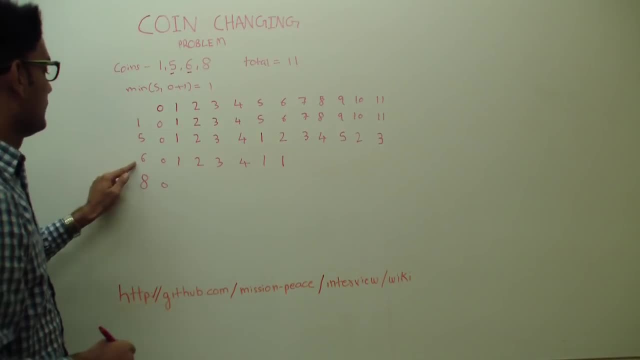 Okay To get 6.. We'll use 1. Again, Because we go back 6 here, We get 0.. 0 plus 1 is 1.. Alright To get 7.. We'll go back 6 here. 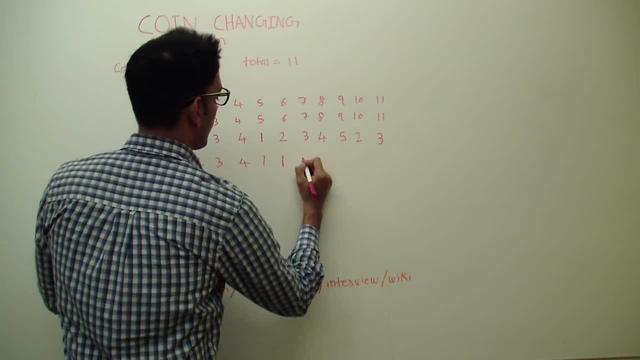 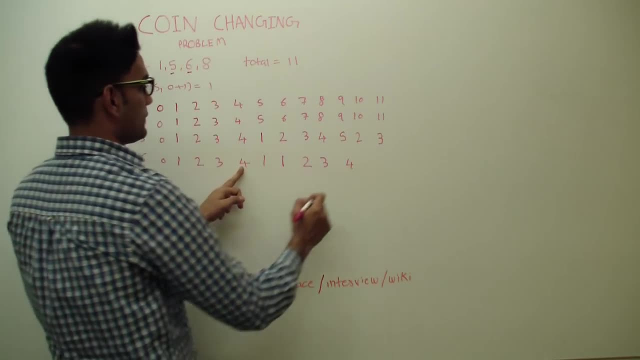 So either 3 or 1 plus 1,, 2. So 2., So 3. 4. So, instead of doing this, we'll pick a value from the top too, And finally we'll go back 6 from 11.. 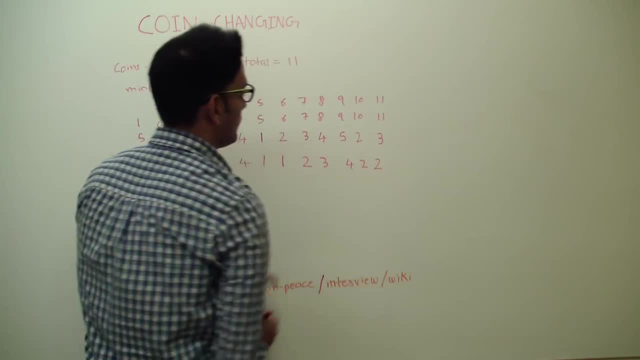 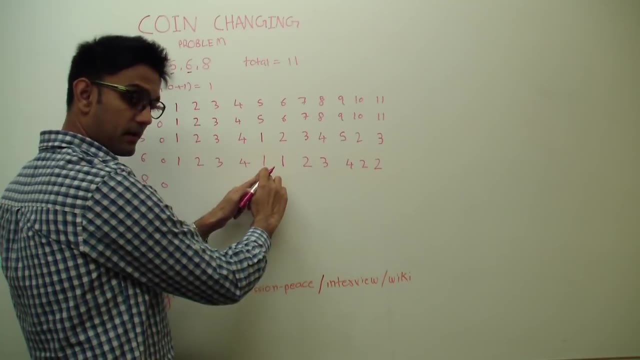 So 1. Plus 1, 2.. So how did we get this 2?? We go back 6 from here: 1, 2,, 3,, 4,, 5, 6.. So 1. Plus 1 coin of 6.. 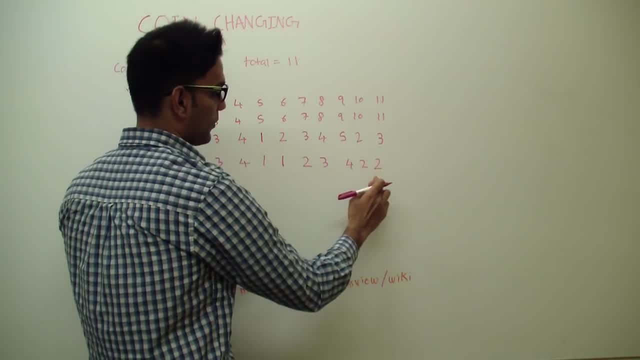 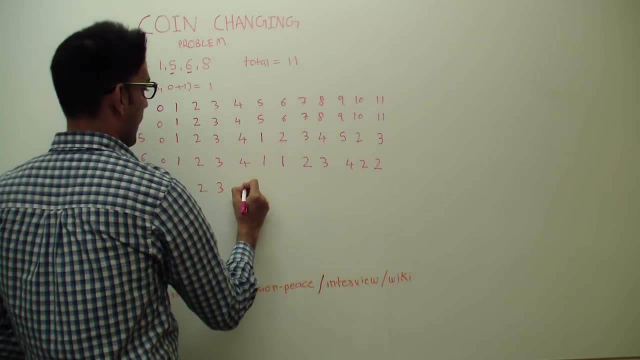 So 2.. So either 2 or the guy from the top Minimum of the 2, which is 2.. So we'll keep 2.. Let's start for 8.. So up till 7,, 8 is going to be same. 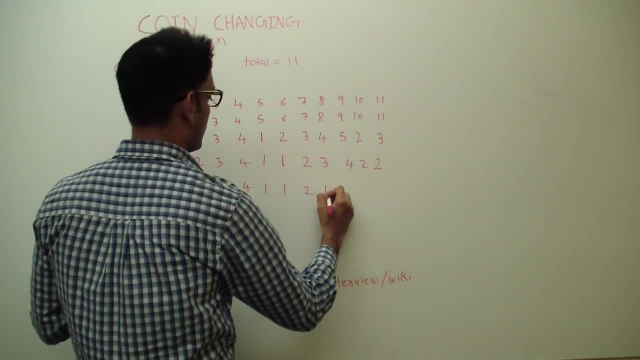 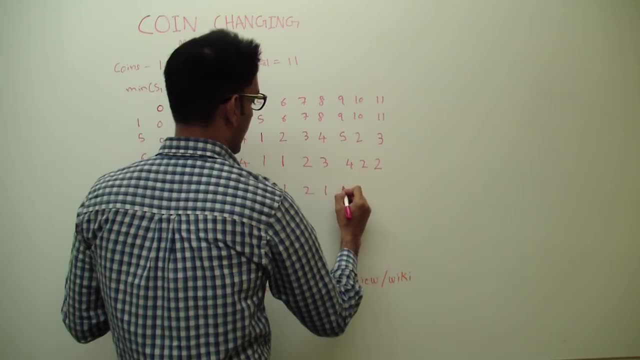 So for 8. We'll need 1 coin, So 1.. For 9.. We'll say 2. Because we come back 8 steps, So 8 plus 1., So 2.. For 10. We'll say 3.. 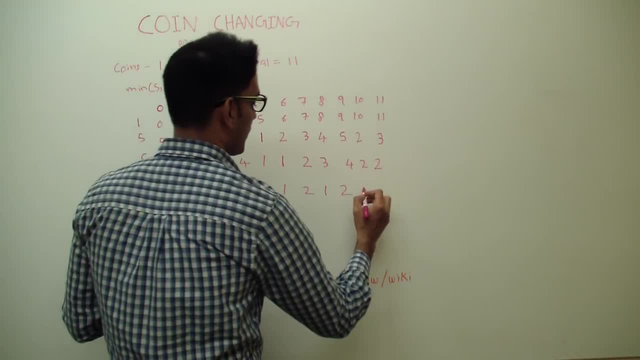 So 2 plus 1, 3 or the guy from the top. So we'll use the guy from the top, So 2.. And for 11. We'll either say 4 or the guy from the top 2.. So 2.. So the final answer is 2.. So, given coins of denominations 1,, 5,, 6 and 8. And given a total of 11. The minimum number of coins we'll need is 2.. 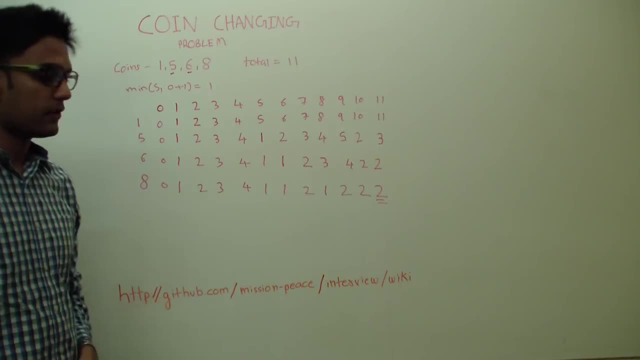 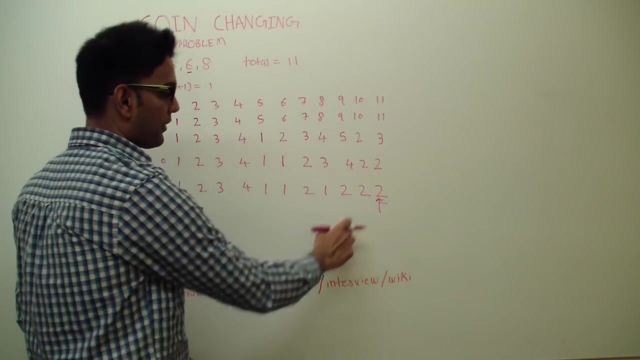 Now, if someone asks you: what are these coins, How do you get the answer? So we'll start from here. We'll say: where is this 2 coming from? Is it coming from the top or is it coming from this side? Clearly, it's that this guy is coming from top. 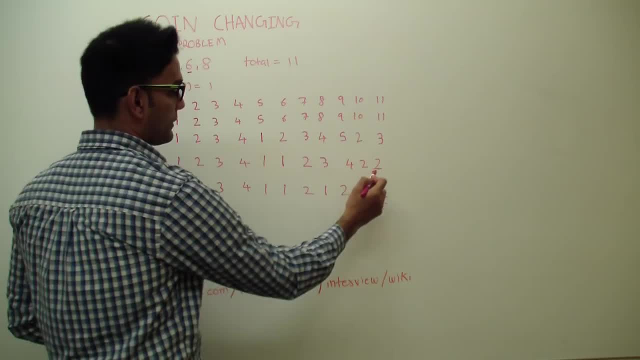 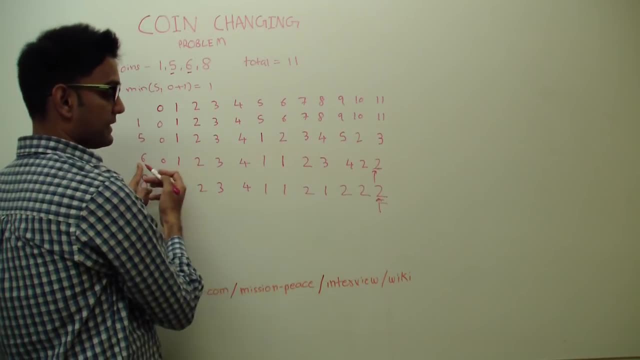 So we go up here: Where is this 2 coming from? This 2 is not coming from the top, So this 2 has to be coming from somewhere here. So we know that 6 is at least in the answer, So 6.. 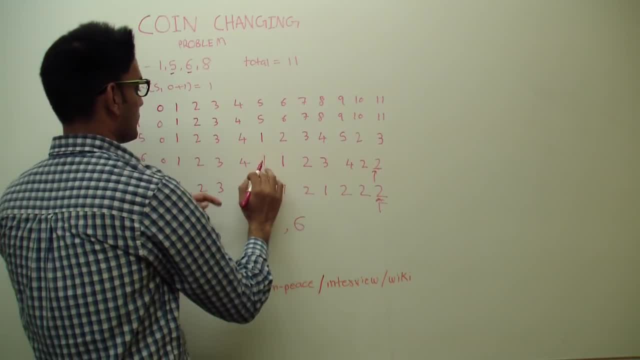 And we go back 6 steps from here: 1,, 2,, 3,, 4,, 5,, 6.. So we are here. Where is this 1 coming from? This is clearly coming from the top, So we go here. 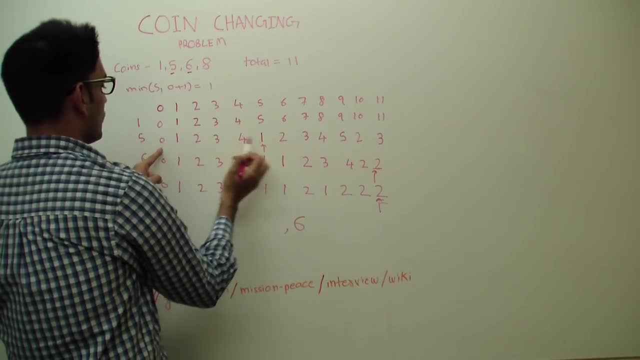 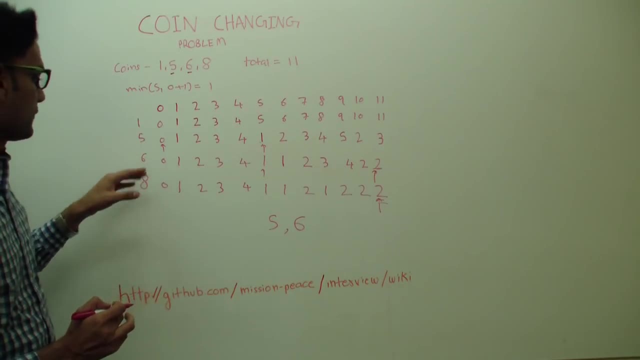 Where is this 1 coming from? This 1 is not coming from the top. So we go back 5 steps here And 5. And as soon as we reach the 0th column, we are done. So our answer is 5 and 6.. 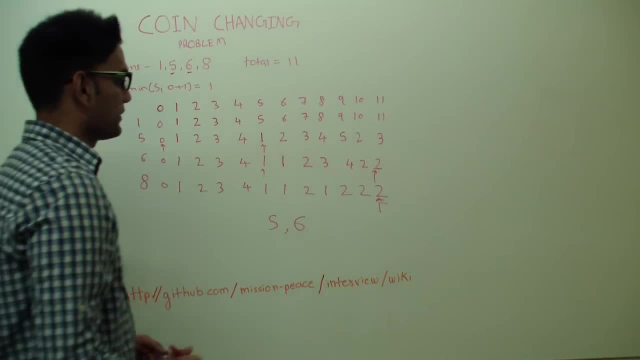 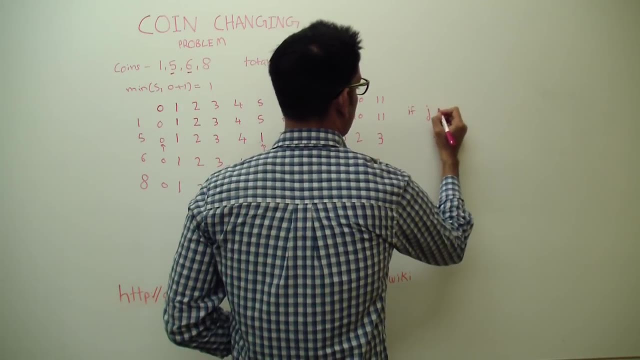 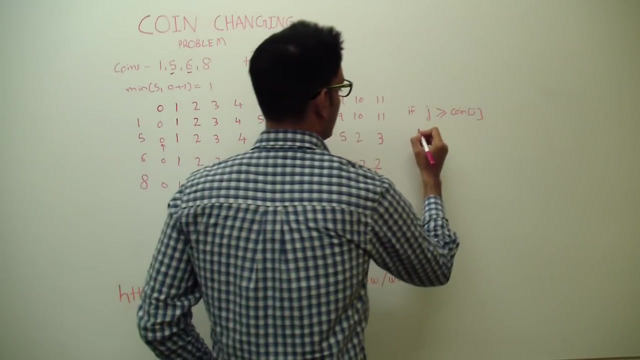 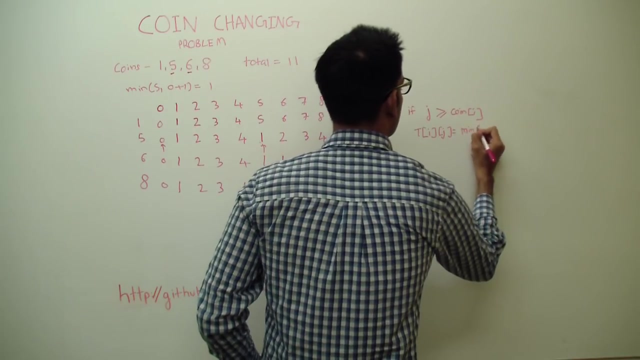 Alright, So let's write the formula for this one. If j is greater than or equal to coin i, then t of i? j is equal to min of t of i minus 1. then t of i? j is equal to min of t of i minus 1.